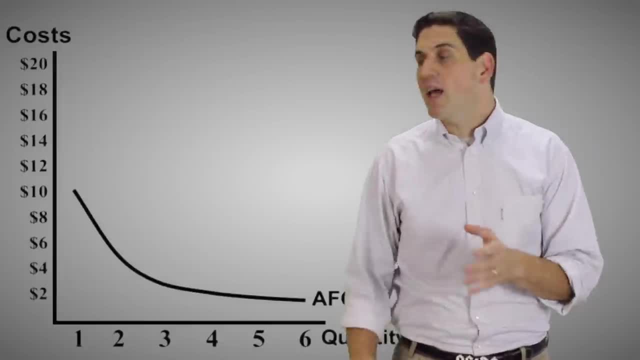 Notice how it keeps getting smaller and smaller and smaller. It's an asymptote. That's because you're taking the fixed cost, which is a set amount, and dividing it by larger and larger quantities. The average fixed cost is going to keep getting. 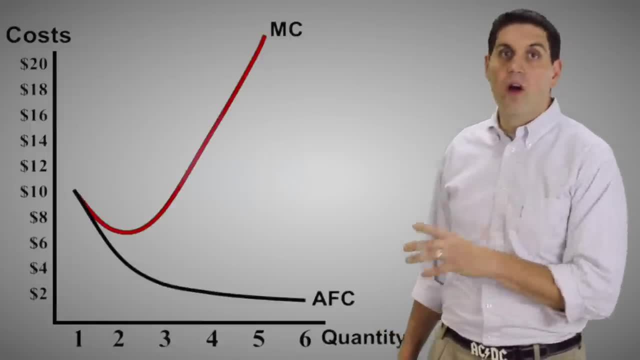 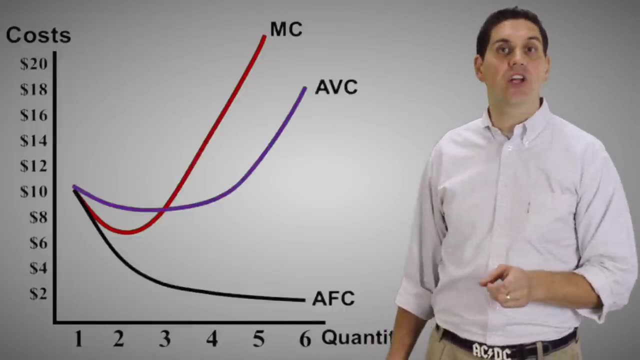 smaller and smaller and smaller. Next up is the marginal cost curve. Marginal cost always goes down and up because the law diminishing marginally turns. Average variable cost goes down and up and it hits marginal cost at average variable cost minimum point. The average total cost also goes. 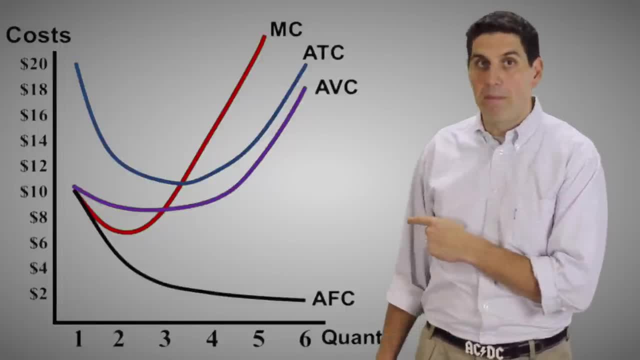 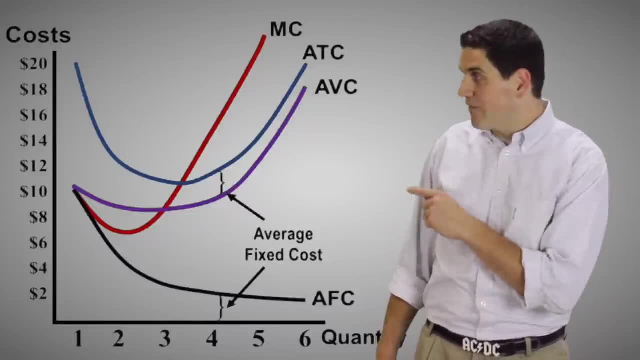 down and back up and it hits marginal cost at ATC's minimum. Notice the vertical distance right here is the same as the vertical distance right there. That's because the average fixed cost plus the average variable cost equals the average total cost. Now let's talk about how you're. 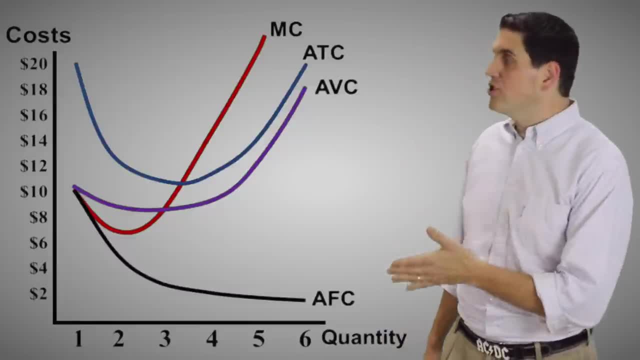 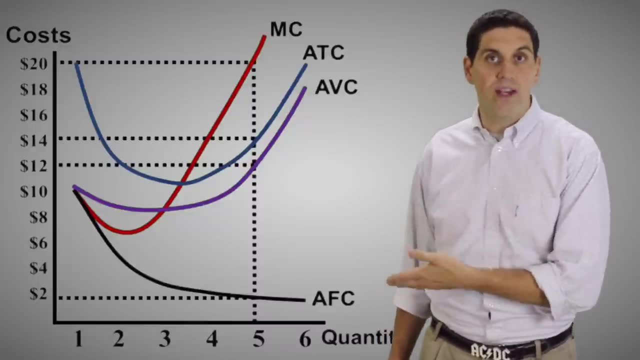 going to actually use this graph. You might get a question on a test that says how much does the fifth unit cost? To figure that out, just go straight up from five units. The graph tells you the marginal cost of producing five units is $20.. The average total cost of five units is $14.. 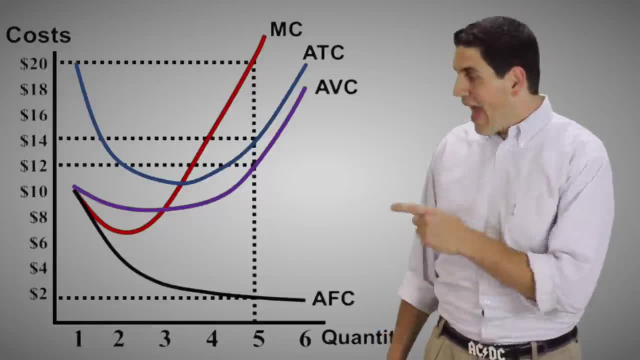 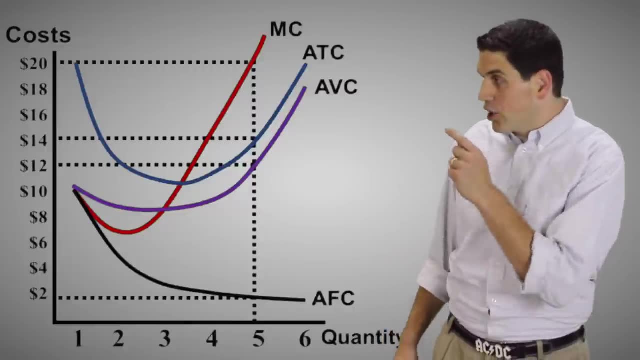 The average variable is $12 and the average fixed is $2.. Again, remember, the average fixed of $2 plus the average variable of $12 equals the average total of $14.. But the best part of this graph is the fact that you can use it to calculate total cost. You can use it to calculate total cost. 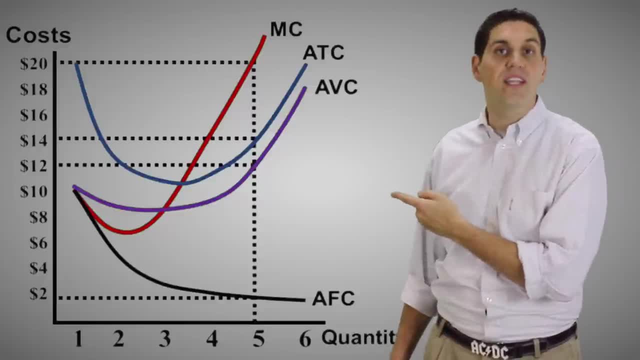 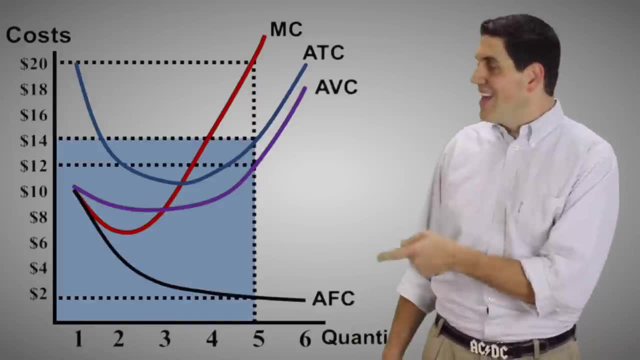 for example, you know that each one of those five units cost $14 on average. Well, how much does five units cost in total? What's the total cost of five units? Well, it's $70.. It's that box right there. 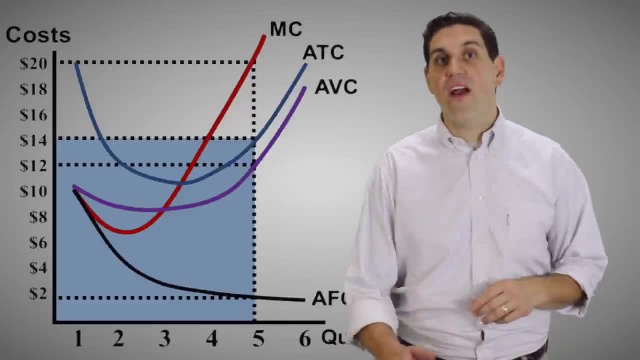 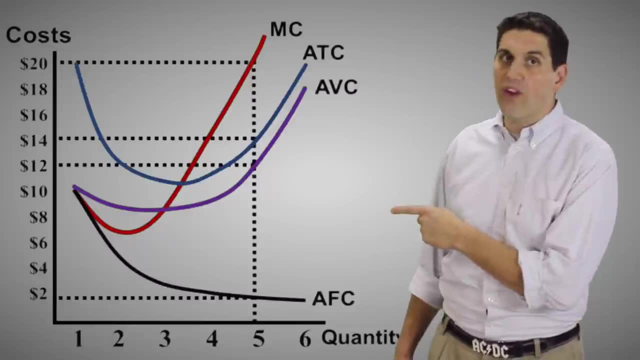 That's the total cost of that $70.. How much is variable and how much is fixed? To figure that out, all you got to do is go up to the average variable cost at five units, which is $12.. 12 times five is 60. So that box right there of $60 is the variable cost of producing five units. If 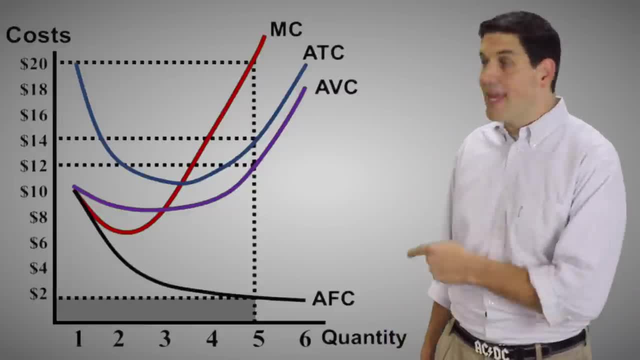 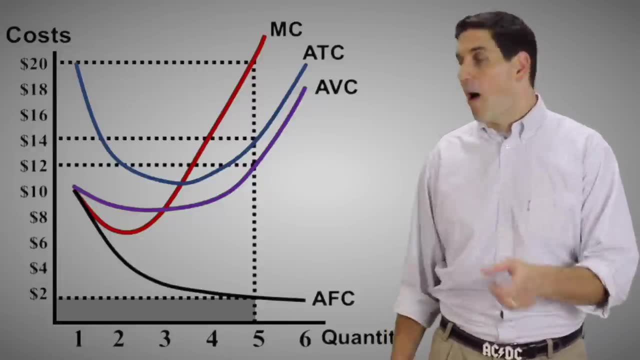 the cost is 60 and the total cost is 70, then the fixed cost must be 10.. That's the average fixed cost of $2 times five units, gives me $10 of fixed costs. That's the box right there. Yeah, All right. 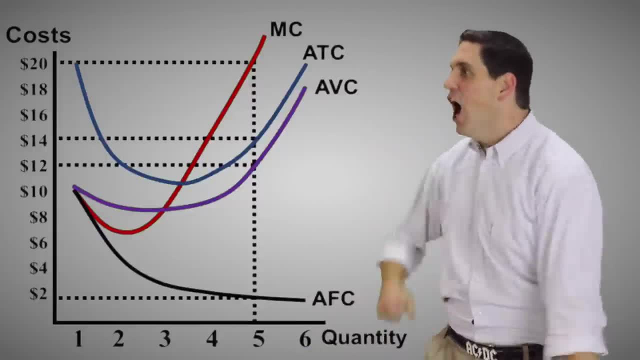 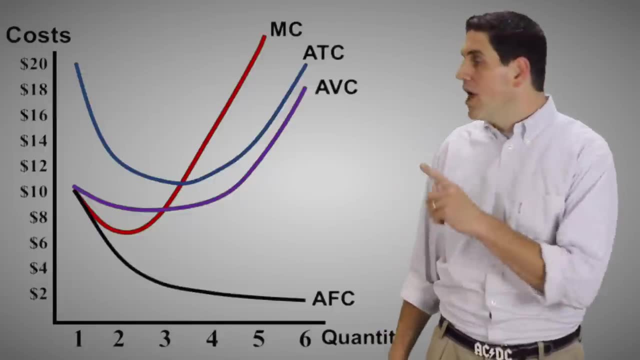 I kind of like this. I'm getting into cost curves. I kind of like it. Yeah, Cost curves, Woo, Cost curves, Cost curves, Cost curves. You're going to be using these cost curves a whole lot, So feel very comfortable calculating the total variable and fixed costs. What you're going to find out.